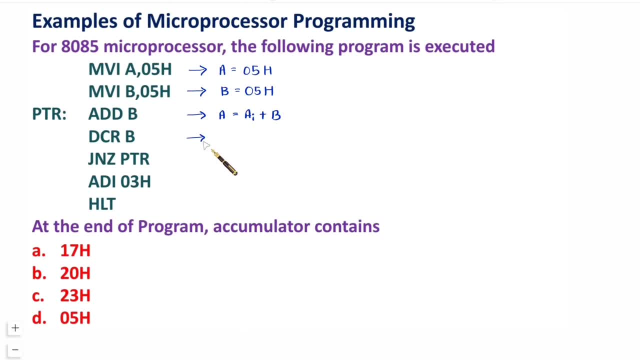 get added with B. So initial value of accumulator that will get added with B and answer will get stored in A. After that we will decrement B. After that we will jump in this loop till that B is reaching to 0. And after that we will be adding 0, 3 hex data with accumulator immediately. So 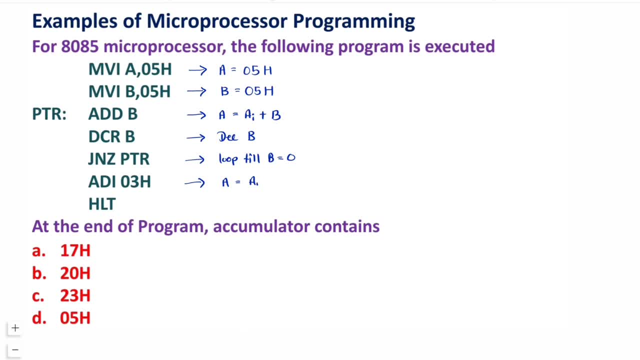 here we are delayed to add initial value of accumulator with 0, 3 hex data And at last time we have added 0, 3 hex data And we also have to add initial outcome. So here, as we have added boolean at the last distance, that initial outcome of B is 0, 3 hex with 0, 5 hex. and this is the end of training. that will now be porridge for all. Après this, we have to write a formula. We are in this process of adding weight thesewand reaching out little part of cumulative rate, ambient in answer period, that is, to what we have discussed previously in this. 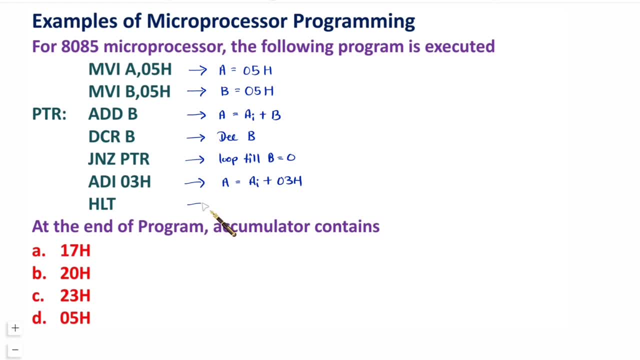 end and for that question, we are now a minute. sometime Now, let me repeat, all these phenomena will be in contact with all. So now, if you danke, last halt is there, So we will be ending our program over here. So now, my dear students, 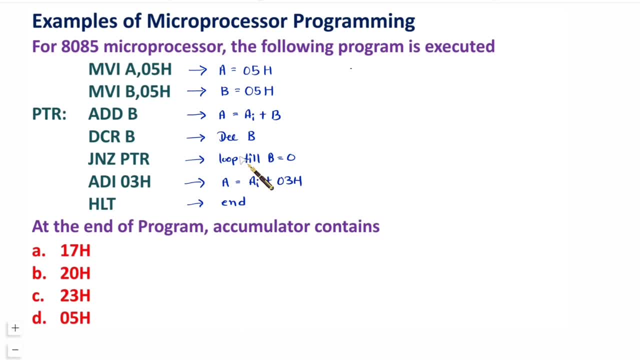 let us see step by step what will be the value of accumulator at the end. So, as I have told you, initially it is phi by mvi a comma 0 phi. after that, b value will be also phi. after mvi b comma 0 phi. after that we will be adding b till that b is reaching to 0, right? So 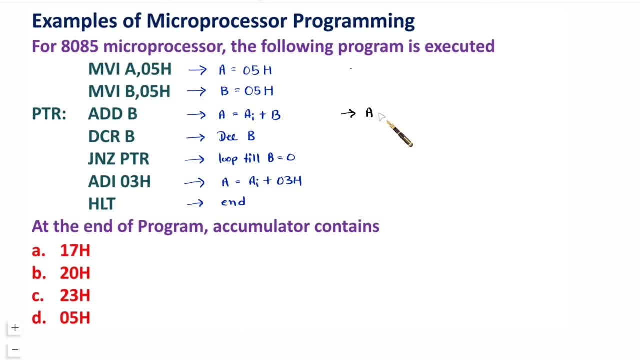 what is happening here? you see here accumulator data. initially that was phi, right Now. initially it will add b, so it will add the value of b. that is phi over here Now. you see, b value will decrement by 1. And it will be having jump if not 0.. 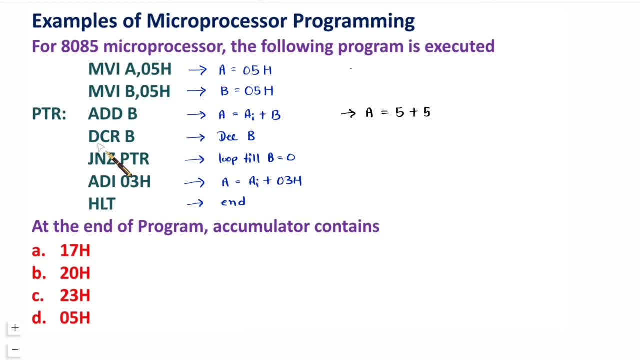 As b is not 0, it will jump it over here Now. next time b's value will be 4.. So 4 will get added Now. that loop will get repeated till b is 0. So 4, then 3, then 2, then 1. that will get added with accumulator. 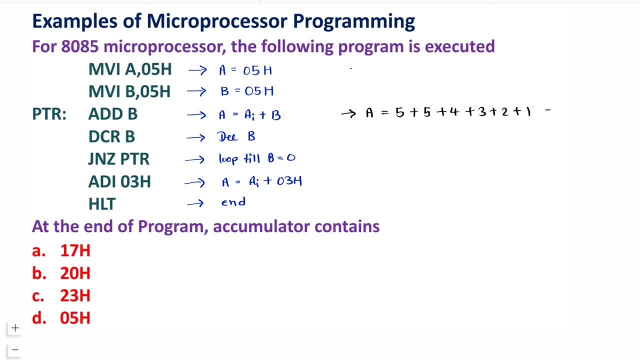 So whatever value of accumulator that is there over here, that is 5 plus 5,, 10, then 14,, then 17,, then 19 and 20.. So this will be 1,, 4 hex. 20 means in hex it will be 1,, 4 hex, right. 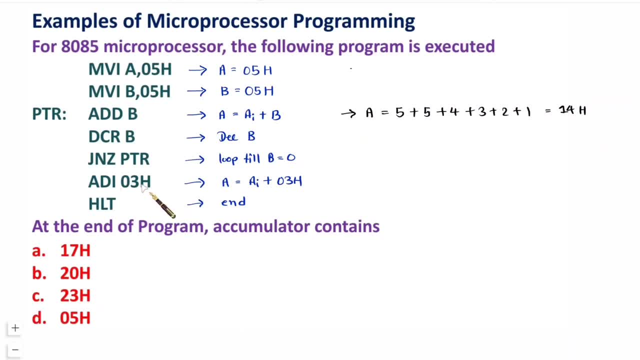 Now this loop is getting executed. After that it will add 0, 3 with accumulator. So here accumulator data: now that will be 14 hex plus 4. 0, 3.. So this will make it to 1, 7 hex. 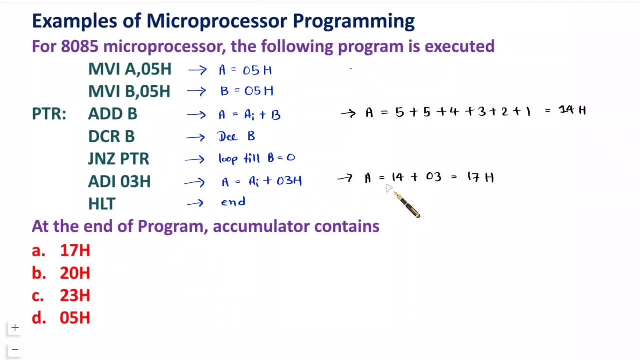 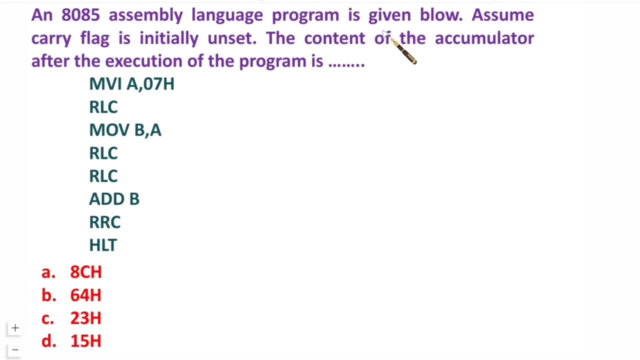 So, after execution of this program, you will be having accumulator that is 1,, 7 hex. So your answer will be this: Now, my dear students, I'll be explaining you. second question: Now here, my dear students, an 8085 assembly language program is given over here. 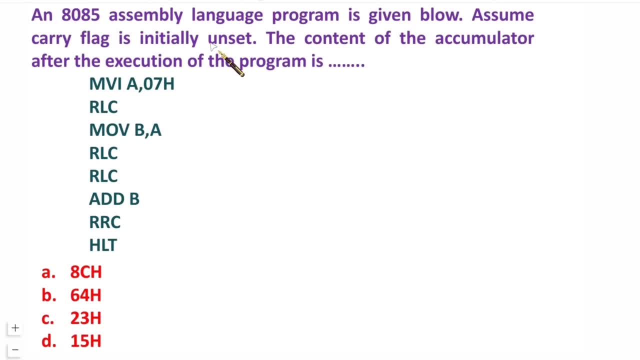 Assume carry flag is initially unset means carry flag is 0.. Assume carrying on is initially unset, means carry flag is 0.. Our decoder rotate accumulator left will happen without carry right. so here we will be rotating left accumulator without carry. after that we will be copying the value. 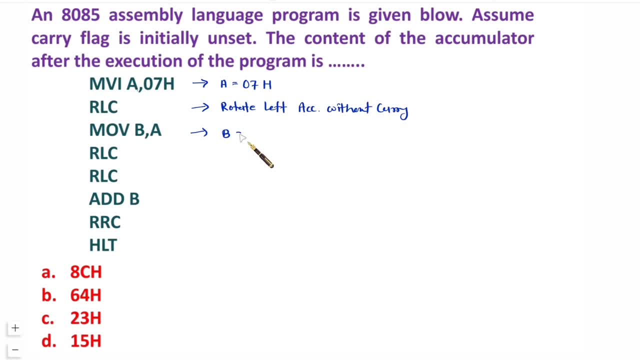 of a into B. so now B will be equals to a. over here. then, my dear students, I'll be rotating accumulator left without carry two times. then, my dear students, here we will be adding the value of B with a and answer will get stored in a. so initial value of accumulator that will get added with B. 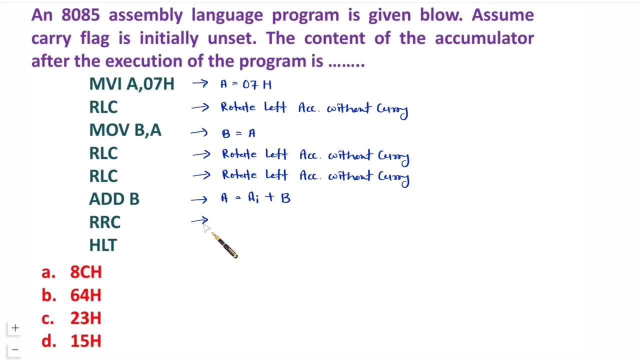 and answer will get stored in a. after that we will be routing the content of accumulator in the right direction, without the carry, and after that we will and our program. so, my dear students, let us see how content is getting changed with respect to execution of instruction. so, first of all, 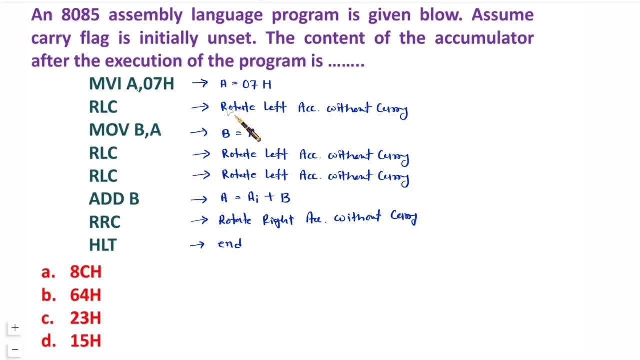 the content of accumulator, that is, 0, 7 hex. after that we will be rotating accumulator left without carry. you see, RLC means rotate accumulator left without carry, and if it is written RAL, then with carry, we need to rotate accumulator left without carry, and if it is written RAL, then with carry, we need to rotate accumulator left without carry. 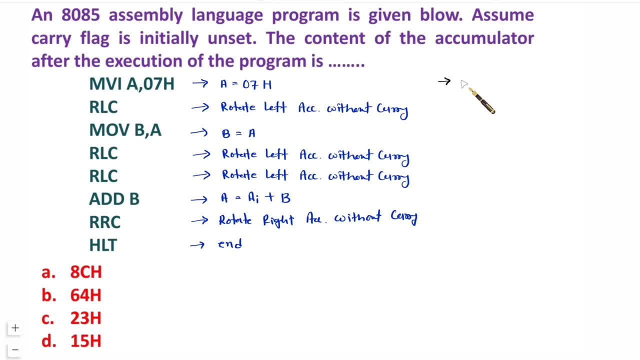 in the right direction. yes, now that is a look good. right, I can count here- there is a little mistake that I found this slide. it get checked the time of Frauen early right now, because Instrbrig sagte: mana power x times i x needs to an take in distance. So that's it. you should read that from B box to B box to the nik本当 term. yeah right, ya, you should know that. so now here, bit by bit, I need to represent initial value of a cphim later. so 0, 7 means 40 sura there and 70這是 011. so that is how we have accumulator initially. 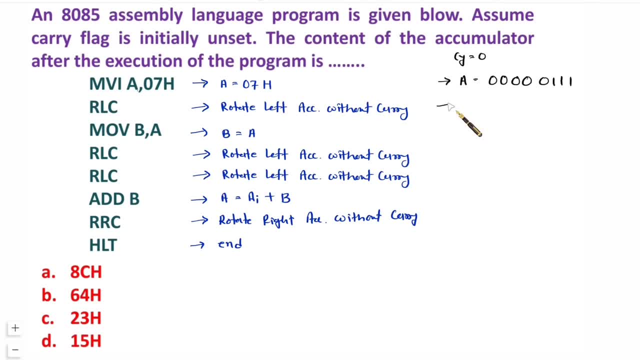 and I have twenty four zeros are and seven is zero, one one one. so that is how we have our Toe. that is collo wheat. buy an extra set and here carry is initially unset. so in a to right. see what will happen here. it will be rotating accumulator left without the carry right. 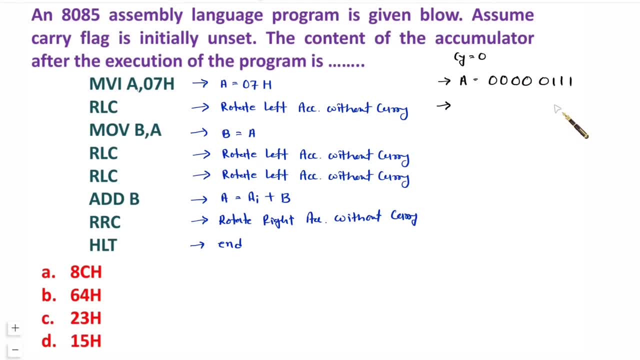 so here you see, this 0 that will come here and this data that will get shifted in left direction. so 1, 1, 1 and then 0, 0, 0, 0. that will be the content of accumulator once you rotate left, right, without the carry and this initial bit that will go in carry. so now carry, that will 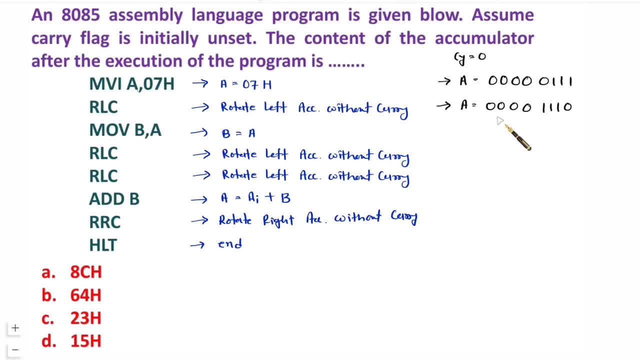 be equals to 0 again, right? So I am not writing: carry is 0, only right now here, move b, comma a. what it does it will be copying the value of a into b. so now, after execution of this, now b is equals to a, and what is a? you see, it is 0, and then this is e, so b is e. 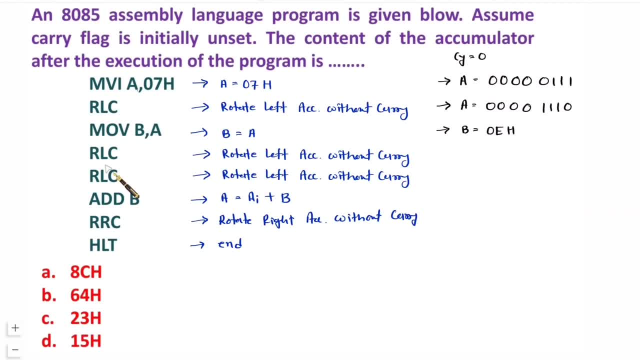 0. e hex, now we are delivered. to rotate accumulator left without carry two times right. so this is what the content which is there with accumulator. if you rotate this by left, you see this: 0 that will come here first and then these are the bits that i need to rotate it towards left side. so again, 0. 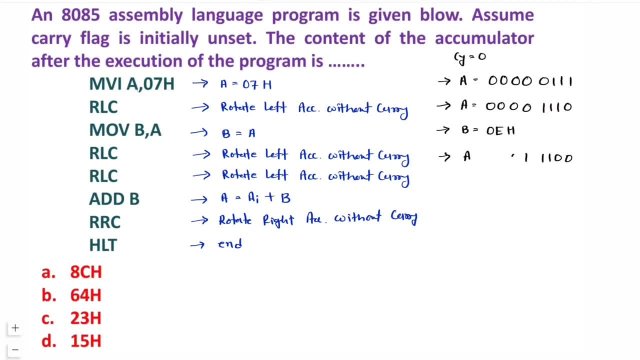 then three ones are there and then three zeros are there. that is what the content of accumulator once you rotate it left once again. if you rotate this towards left side once, then this 0 that will come here, so this 0, and then this 2, 0 that i need to write. then triple 1 is there, so 1, 1, 1 and then. 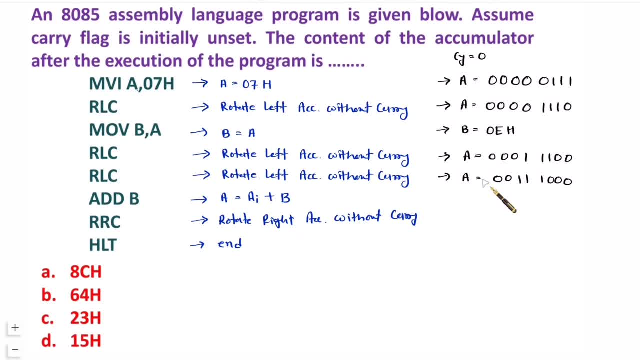 this 2, 0 that i need to write. so this is the content of accumulator once you rotate it second time. After that we need to add b. so here this is what initial value that i can say and this is what 3 and 8. so 3, 8, hex. that is the value of accumulator right now. after addition of 3, 8, x with b is equals. 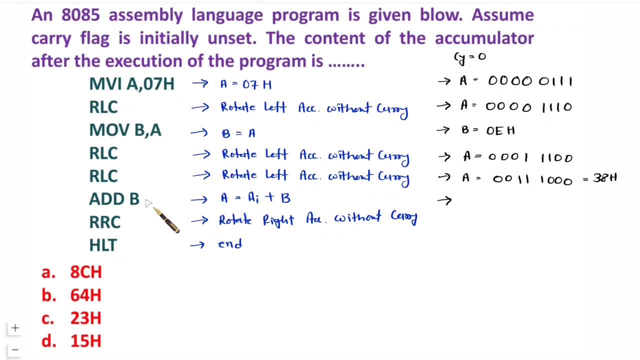 to 0, e will be having that add b operation. so i can say a now that is 3, 8 plus 0, e now e is 14, 14 plus 8, so that will be 22. so if you subtract 16 from 22 there will be carry 1, and if you subtract 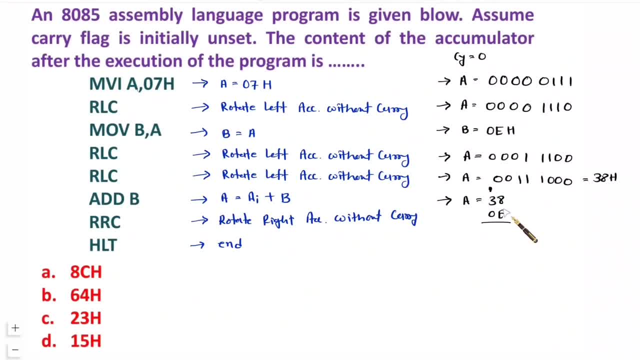 16. from 22 you will be having 6, so i am writing 6 here and here you see 1 plus 3, that will be 4, so accumulator that will be 46 hex. after this, add b. now, my dear students, Again I need to rotate accumulator, but towards right side. 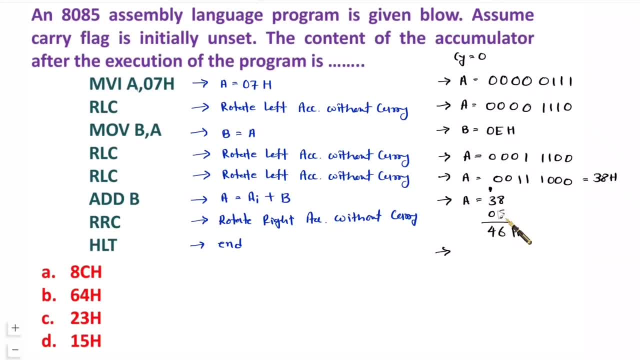 And here you see, after addition, there is no carry right, So carry flag is 0.. So now I need to represent this 4, 6 in terms of bits. So 4 is 0, 1, 0, 0 and 6 is 0, 1, 1, 0. 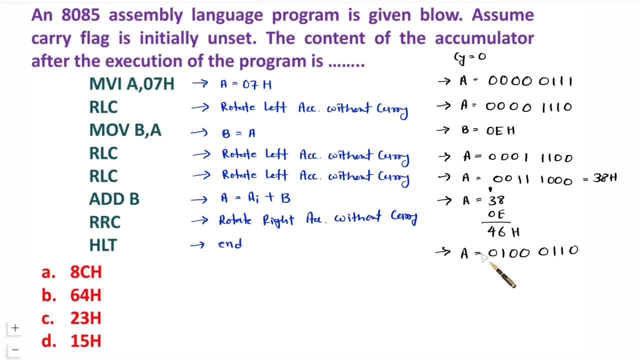 Now I need to rotate this accumulator content towards right side, right. So here see this 0,. now that will come over here and without carry, that we need to rotate right So it will not get affected by the value of carry. 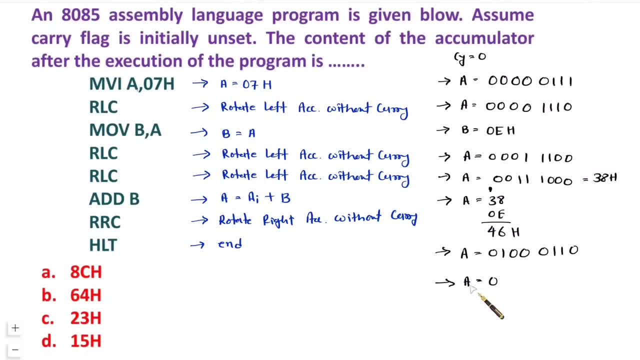 Carry flag will get changed, but data of final answer will not be depending on carry, So this 0 will come here and then you need to shift all this data towards right side. So 0 then 1, then 0.. 0.. 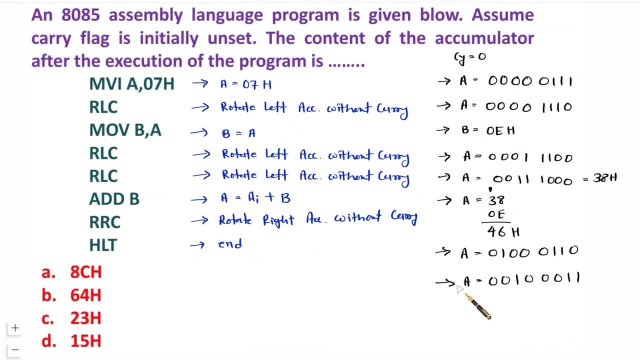 0 and then 1, 1.. So that is my answer of accumulator after RRC and then program is getting ended. So this answer of accumulator that is 2, 3 hex. So answer for this question is 23 hex. 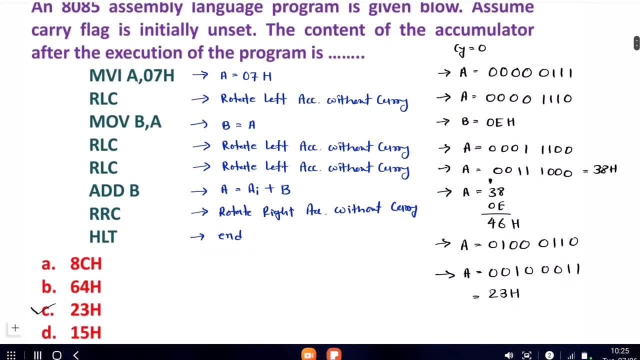 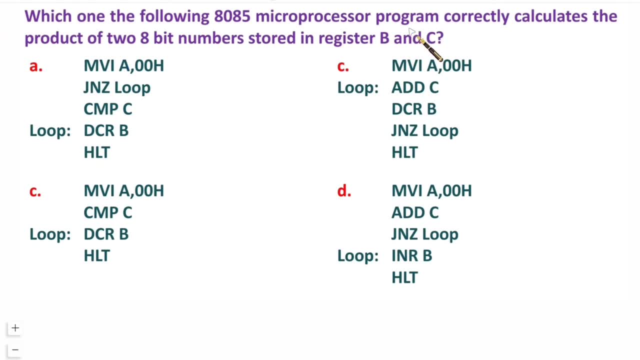 Now, my dear students, let us have third question here. So here, my dear students, question is: which one of the following 8085 microprocessor program is correctly Calculates the product of two 8-bit numbers stored in B and C. So here you will have to identify: product of B and C means multiplication of B and C. 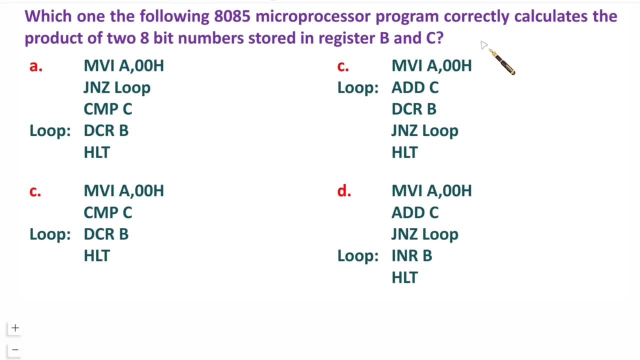 My dear students in 8085, how do we perform multiplication? We perform multiplication by adding BC times or by adding CB times, right? So if you add BC times, then you can say that That is what B into C. 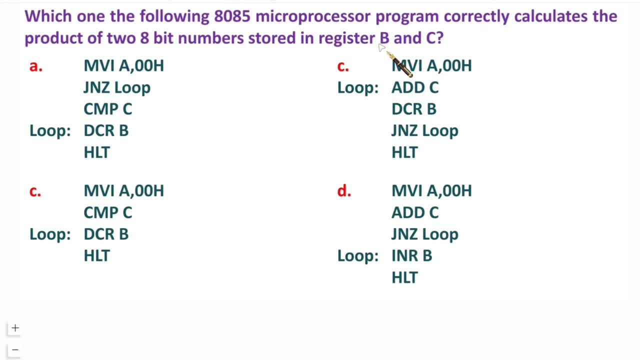 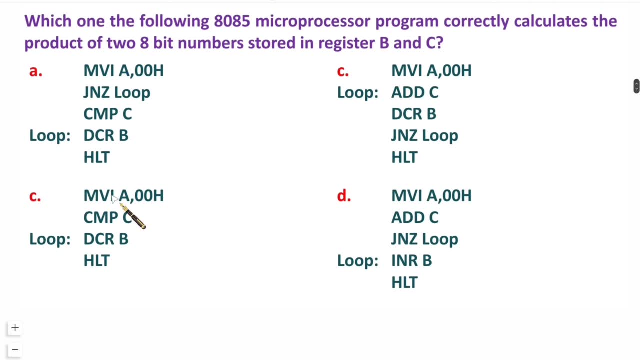 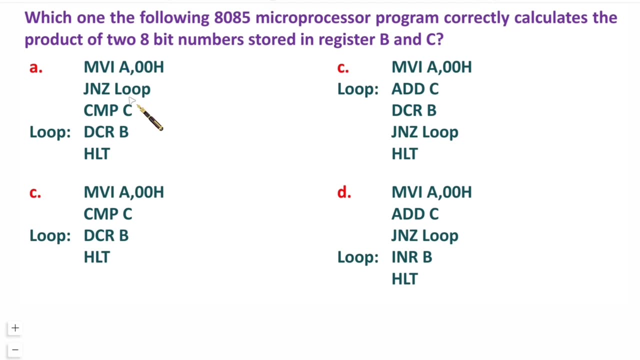 Or as if you add CB times, then also you can say that is multiplication of B and C. So let us check it whether it is happening with these all four possibilities or not. So, my dear students here, MVIA, comma 00, after that jump, if not 0, then loop is written here: 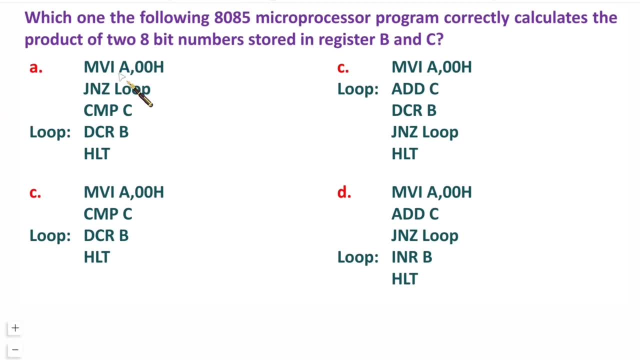 Initially value of 0. that is there with accumulator, So it will jump it over here. Then DCRB will happen and it will, So it will jump it over here. So here there is nothing which is happening in terms of multiplication. So I can say: 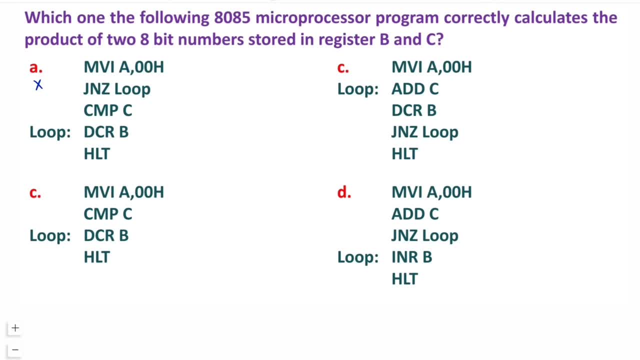 this is my false option. after that here, MVIA comma 0, 0 is there. then compare is been done. So this cannot do multiplication. So this is also false option. Now you see MVIA comma 0, 0. that is there. with this. Now we are adding C initially and we are decrementing B, So